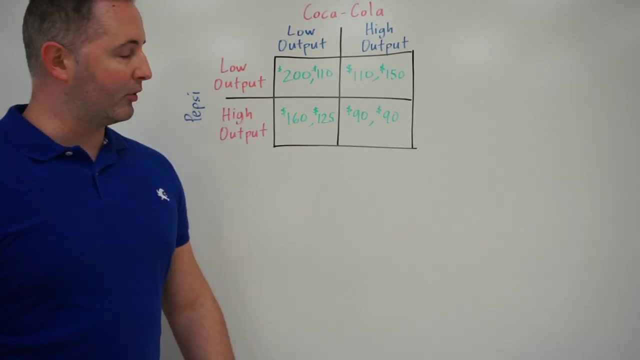 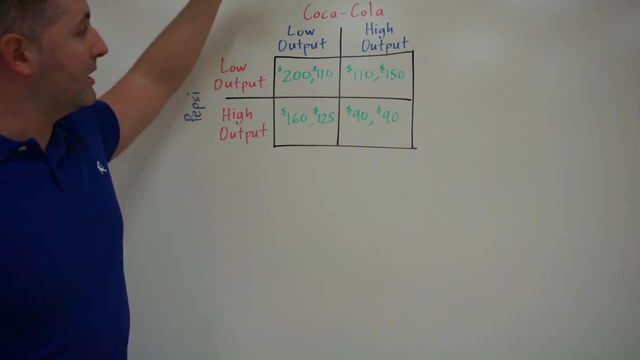 So what we're looking at here is relatively simple. Um might look a little intimidating, but it's not that bad. So first of all, we see that each of them has the same two options, right, Coke can either have low output or high output. Pepsi either low output or high output. 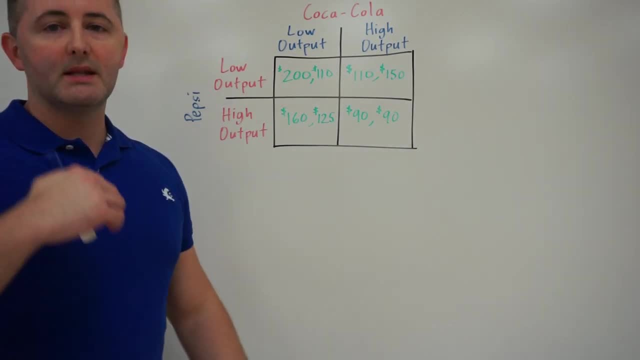 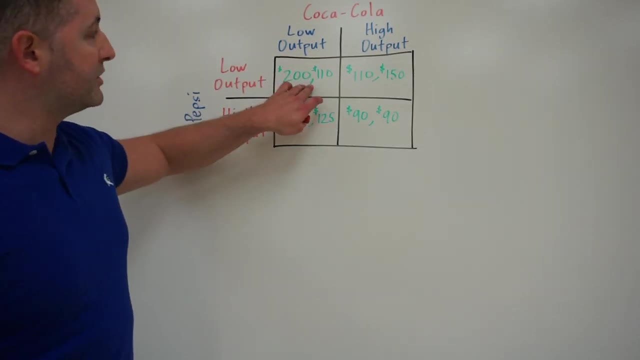 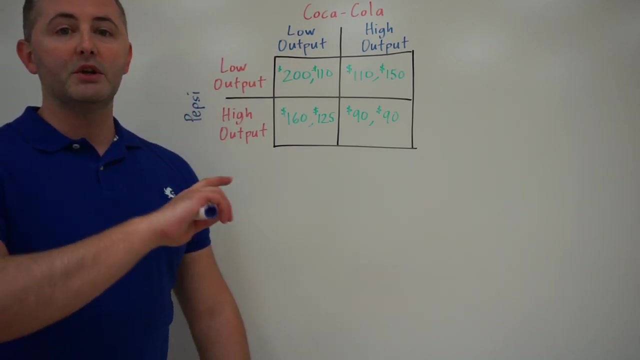 So what do these numbers represent? These represent the profits that each of these firms would make if they choose these two combinations. So this quadrant reflects what happens if they choose a low level of output. Now the important question is: which is which? Okay, So to help us out. 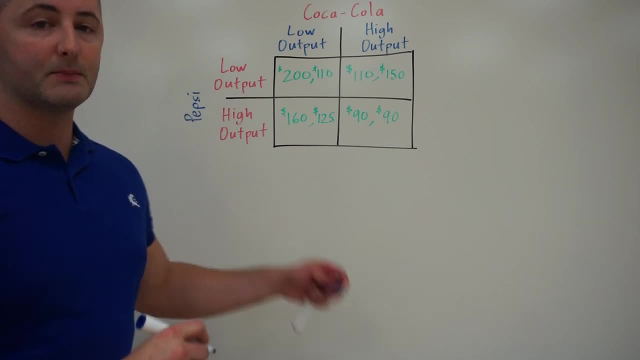 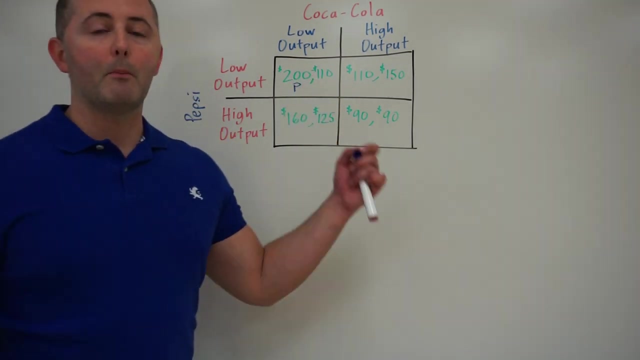 here I'm going to put the letter P or the letter C. letter P represents that that's Pepsi. Um, that's going to be our horizontal axis up. the letter C for Coca-Cola: That's our vertical. All right, So this will apply in every payoff matrix that you do. All right, This number, $200, that is the amount. 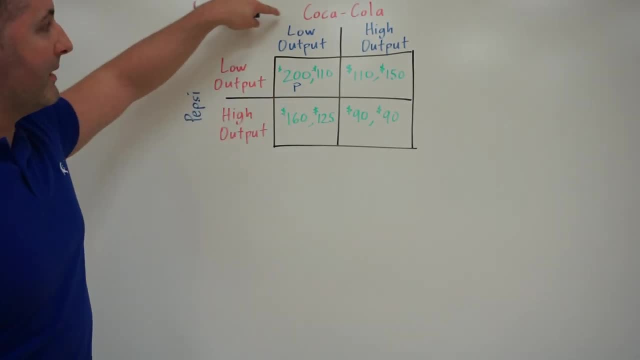 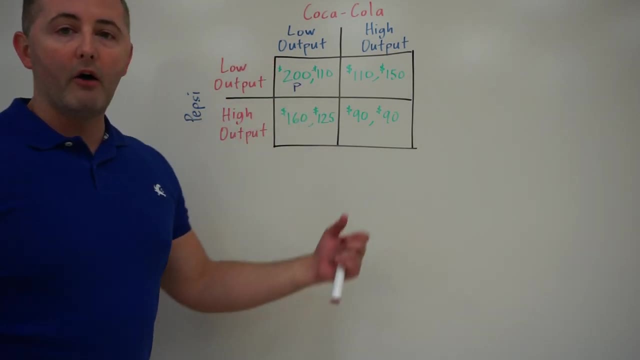 Pepsi would earn, That would be Pepsi's profit, if they both choose to do a low level of output. So the first number, the one on the left, that's always going to be the number of the horizontal axis. So that means if we dropped down to this box with high output, that would be Pepsi, with the 160. 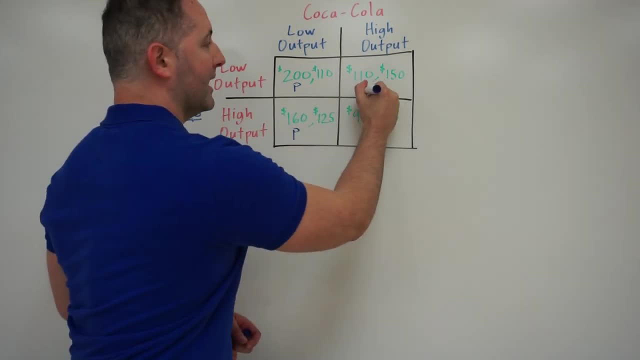 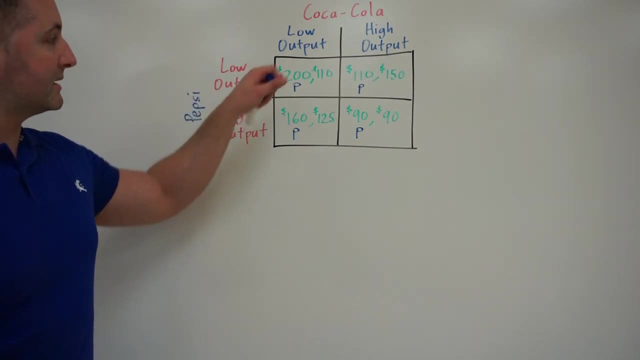 All right, If we move over to the right side, Pepsi would be the first one. Again, they're always on the left. That's the one 10 and Pepsi is the first 90 over here. So our horizontal axis is always the first number left to right in the box. Okay, Coca-Cola, since that's our vertical. 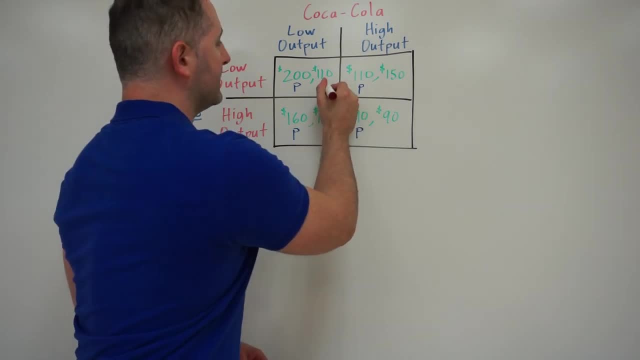 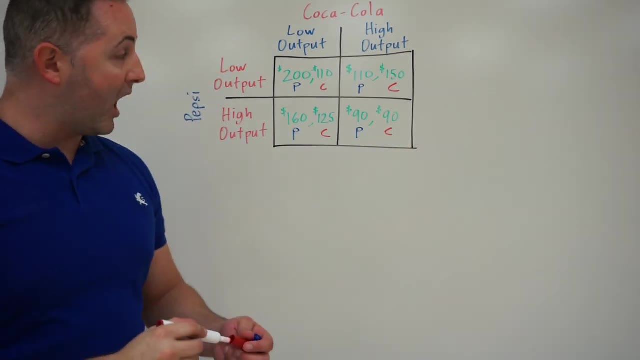 axis. that's always going to be the second number here. So again, it's pretty simple. We walk through it. We have our Coke on the right, Coke on the right, Coke on the right and Coke- you guessed it- on the right hand side. So this telling us, now we can look and we can compare. All right, If they both. 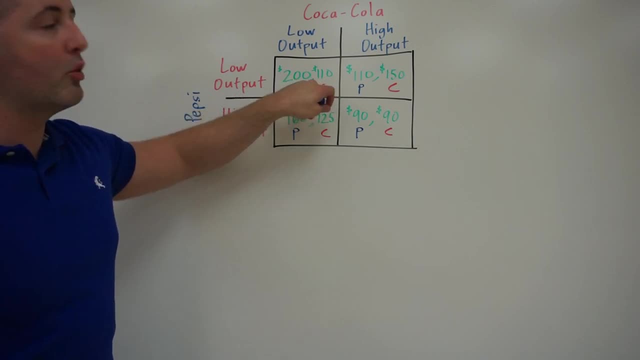 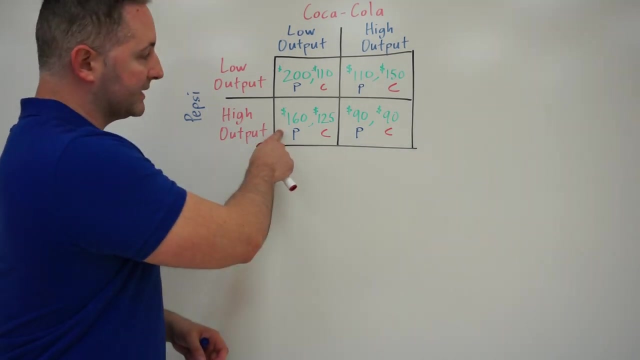 do low outputs, Pepsi will earn $200.. Whereas Coke will only earn 110.. If Pepsi does high output and Coke does low, this will be the combination: Pepsi will earn 160.. Coke will earn 125, et cetera, And we 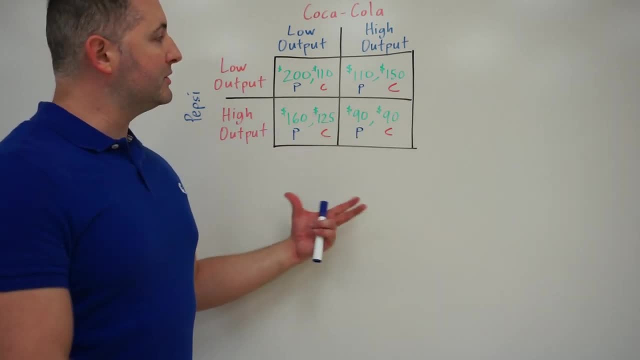 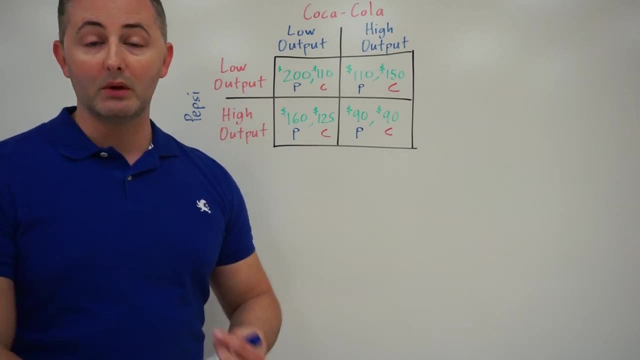 do it for all four combinations. So we're going to use this information to then make certain determinations of whether or not these firms have a dominant strategy, to find a Nash equilibrium, if one exists, and also to determine whether or not these companies find themselves in what is known.